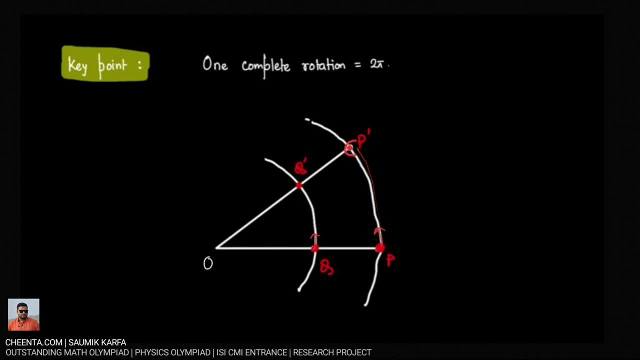 moving on a circle. So we moved P on a circle and this is the new position of P prime. So if we want to measure that, how much the point P has moved, that will be the angle theta. But what is this angle theta? This angle theta is actually the arc length of P, P prime over 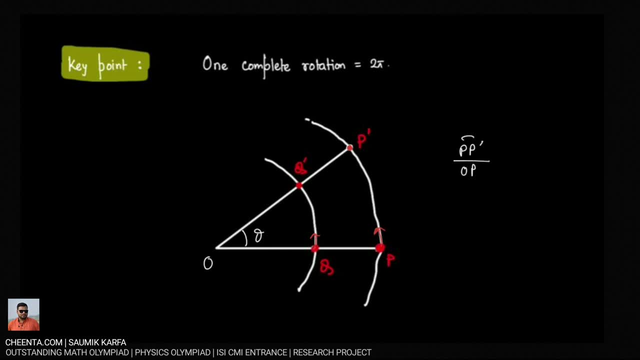 The distance OP. So angle theta is equal to the arc length P. P prime means the distance of point to image over OP, which is the distance between point to center. Now, on this radius OP, any point is moving that same amount because, like if we measure the angle, here also. 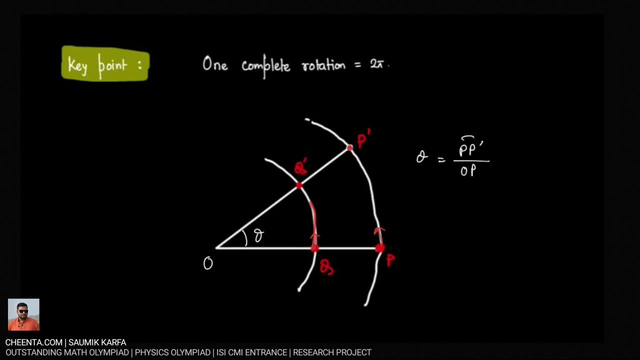 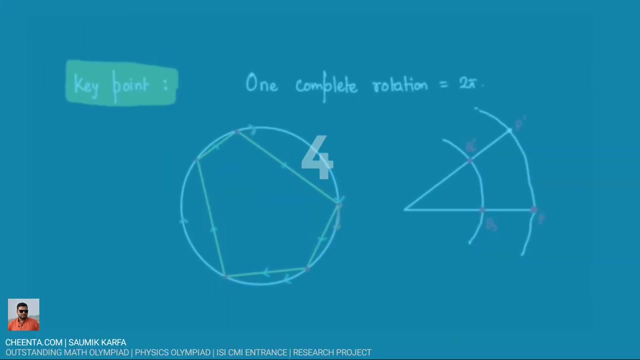 if Q is a point on that same radius, then the movement of Q will be here, which is Q prime. so the angle will be Q- Q prime arc length, Q, Q prime arc over OQ and these two ratios will be same. so in that way angle stays same. Now, if we start on a circle, let's say this is: 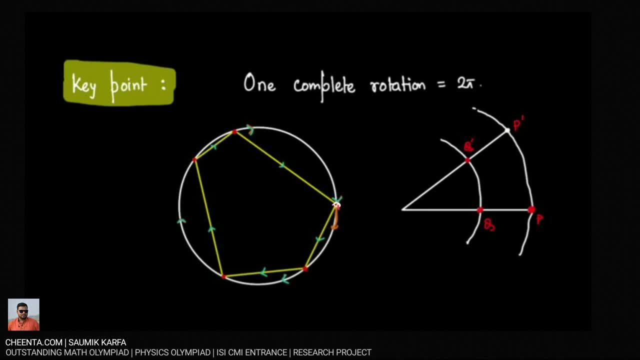 the point P. If we start here and if we start moving on the circle- let's say this is the point P- if we start here and if we start moving on the circle and if we come back to the original position, then the angle made or the amount of rotation made will. 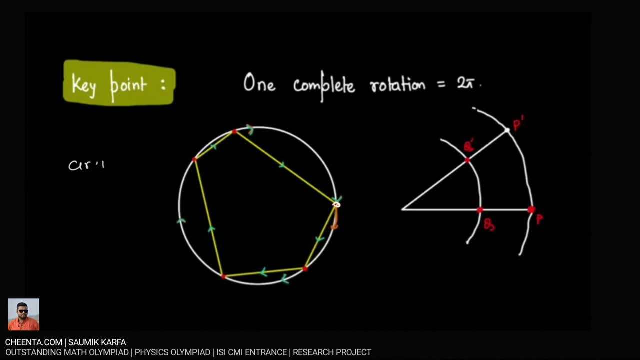 be the circle over the radius or the circumference of the circle over the radius, which is actually 2 pi. So this is taking one complete rotation which is equal to 2 pi. We know circumference of the circle is 2 pi, r over radius is r, so that would be 2 pi. So the same thing can be done by: 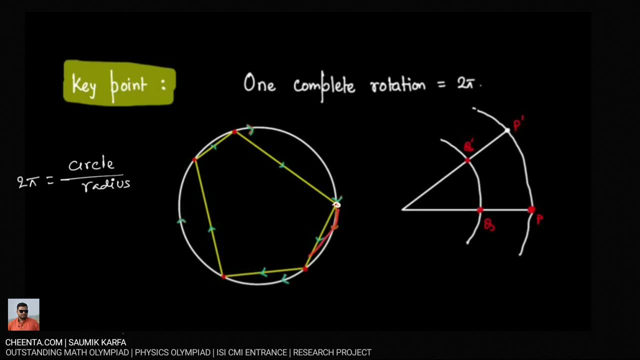 taking some discrete turns as well. When we are moving a circle, moving on a circle, we are taking continuous turn. at every point we are taking a very small amount of turn. but if we don't do that, rather if we first come here by a straight line, 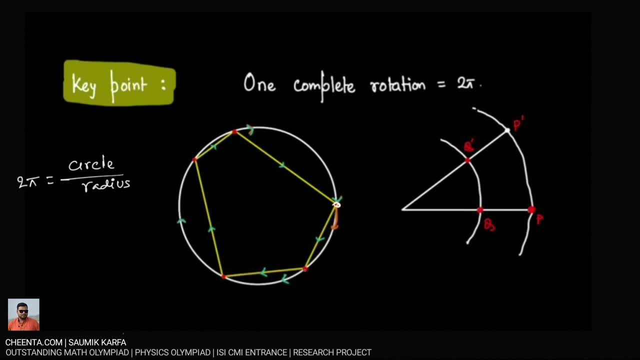 then we are taking a complete rotation which is equal to 2 pi. So this is taking one complete rotation. then we take a turn and come here. so the turn that we actually made is this turn- then if we take another turn- so actual turn we are making is this and so on- if we keep on doing this and we come. 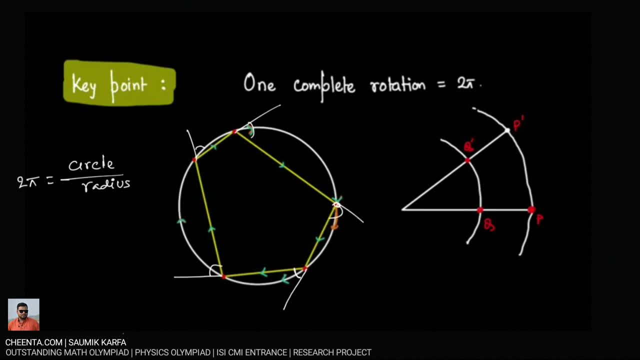 back to our original point and then we face the same way we were initially facing, then that will be taking one complete turn again. So this sum of all these discrete turns must be equal to 2 pi. Now if you notice that these yellow lines creates a closed polygon, So walking through a closed 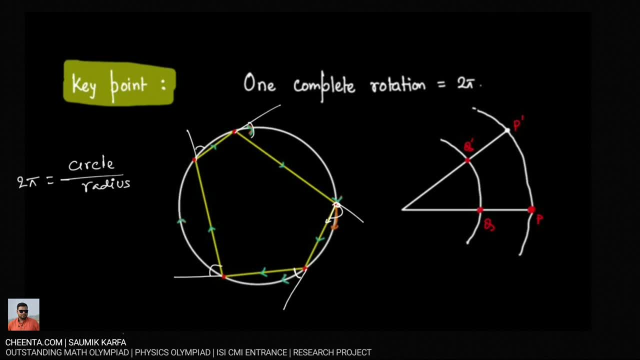 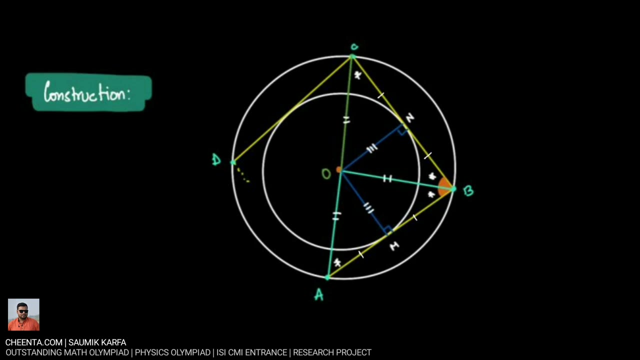 polygon is basically taking one complete turn, and this one complete turn will be equal to all of sum of all of its external angles. So that is the idea we are going to use in the problem. Now let us go back to the problem and start making some constructions. So first of all, we will 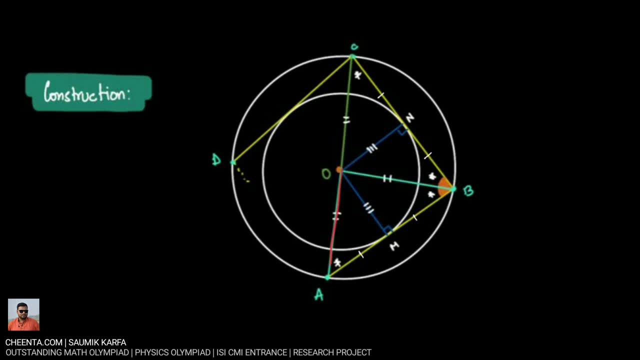 join the center with all of these end points of the chords. and now it is very easy to show that these triangles, where this blue line is basically the perpendicular on this chord from the center, So it is very easy to show that these triangles are basically congruent. triangles means they're. 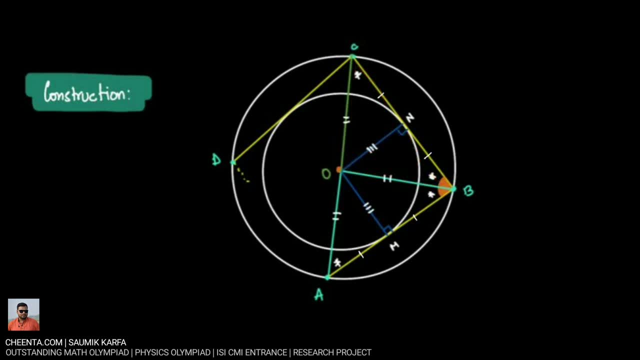 copy of one another. all these triangles are congruent and in that way, we will be able to prove that the angles are congruent. So we will be able to prove that the angles are congruent. So it is very easy to show that the angles are congruent and in that way, we will be able to prove that the angles 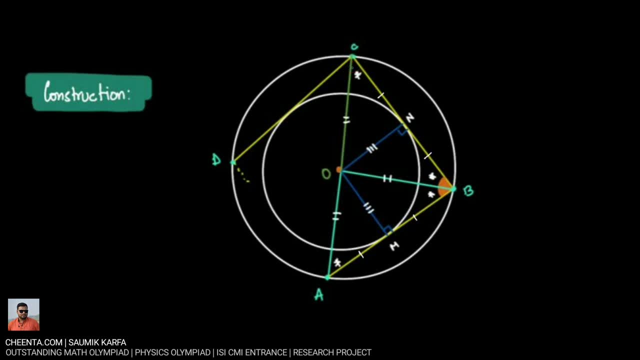 between any two chords, this angle, or this angle, will always be equal. Now, we were given that this angle was 75 degrees, So if we see that this angle will also be 75 degrees, and not only that, whenever we will make such a chord, the angle between that chord and the previous chord will. 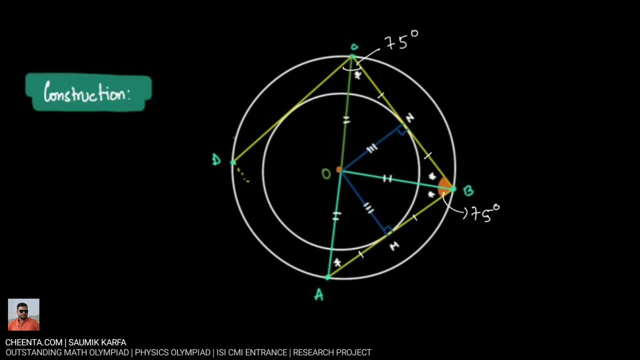 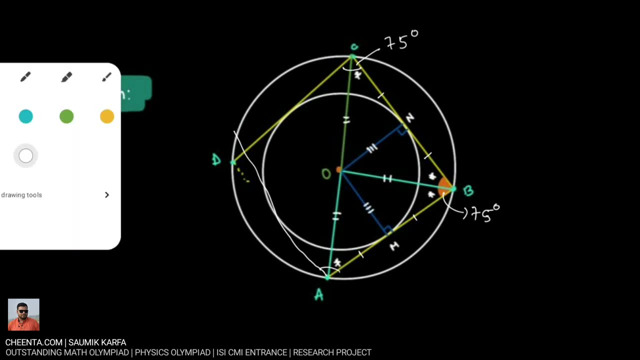 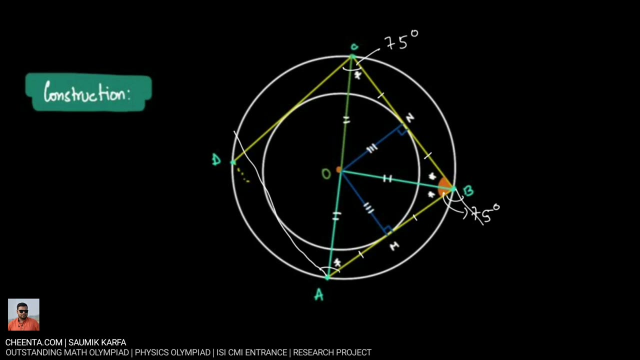 always be 75 degrees. So if we create this chord here, the angle created will be 75 degree. So each time, the turn we are actually making is the external angle, which is equal to 105 degree, and number of such turns will be equal to number.